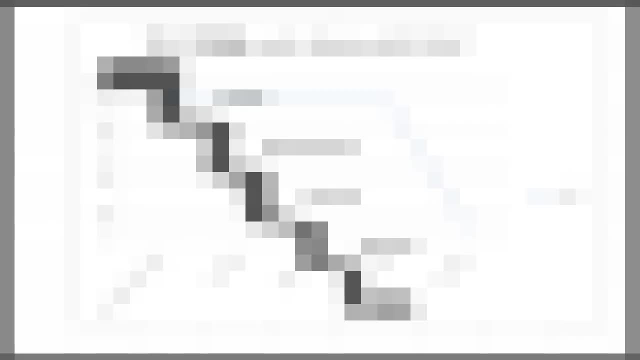 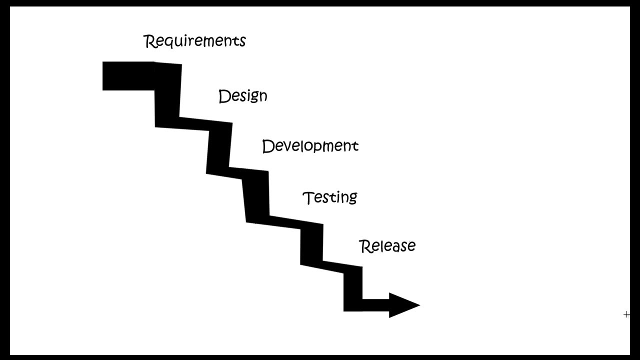 we're focusing on in this installment: The waterfall. The waterfall is very common, It's been used forever, It's simple, It's linear, It's direct Work flows in this direction and it's definitely best suited for short projects only. as mentioned, the risk is too high. 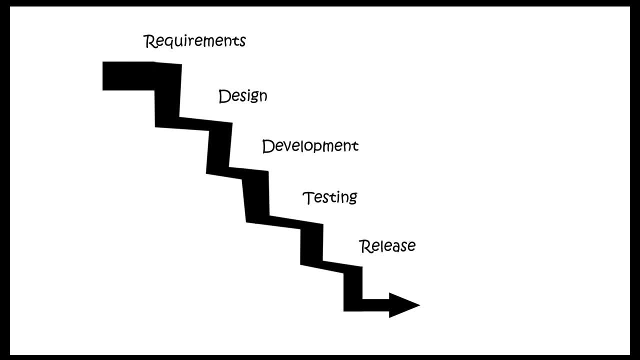 and the cost could be too great for using the waterfall model exclusively over a very large project. consider a few things about the waterfall. the team starts out gathering requirements and the team that's involved in that process consists of stakeholders such as the product definition team, the customer facing team members, business analysts, who are there to document every aspect. 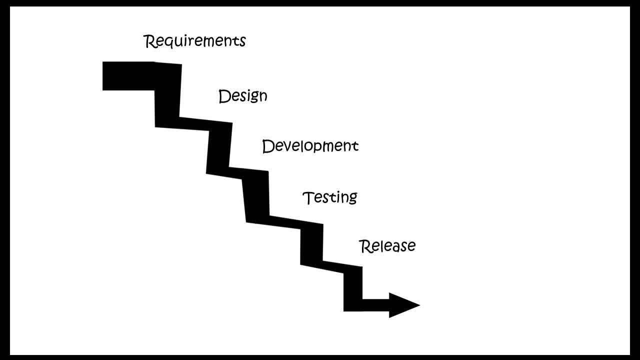 of the functionality that is expected from the software. there should also be representatives from other teams. you might have your development management team there, your testing management team, but at this point during the requirements, you still have not established the complete team. you don't have all your developers, you don't have all your testers, but you do have a core set of. 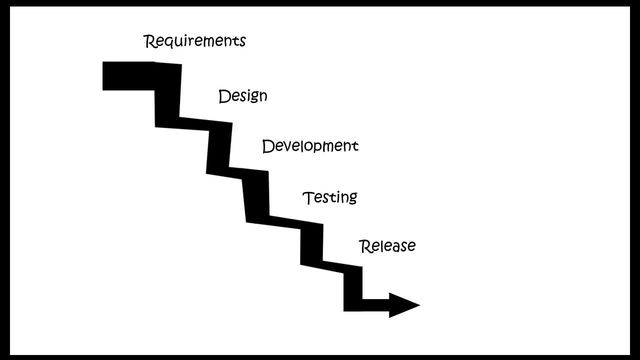 stakeholders who are championing or creating a new product idea. but once the team moves down to design, you suddenly have a need for a different team. you no longer need your business analysts. you no longer need so much your product definition team. the product's been defined, the requirements, 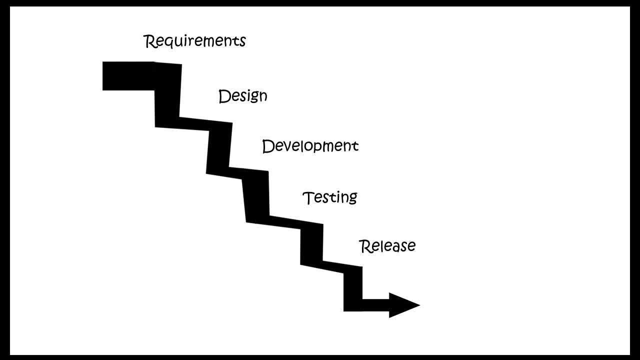 should contain the complete definition of the product that you want to build, and the design layer is then to start to really come up with the physical design of the software. what is the software we're going to build before we go and build it? so we have the blueprint now. 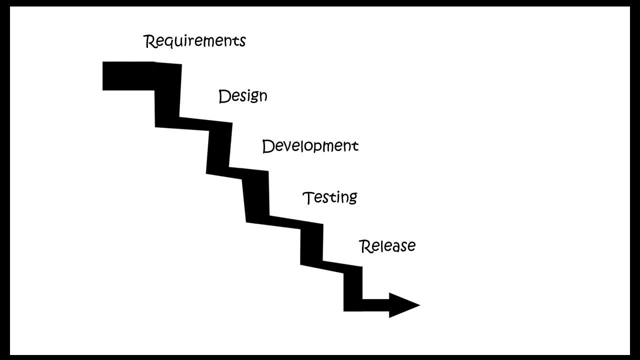 moving from requirements to design and development. i can give you some analogies. it's like filming a movie without a script. it's like taking a trip without a map. it's like cooking a new, complicated meal without a recipe. it's like playing a song without knowing the music. it's like building a 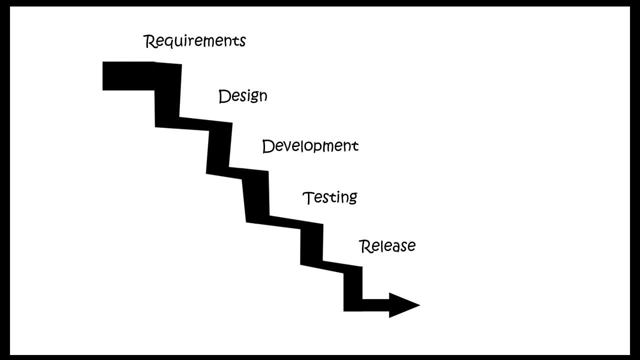 house without a foundation, because that's what the requirements are. they're the foundation of everything you're going to do. from that point on, everything that comes after requirements is going to point back to requirements in some way or another, and there's an entire installment of project management mystery theater on requirements. 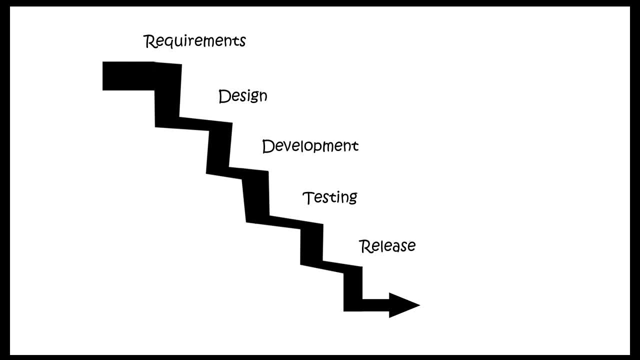 but something to consider about the waterfall model: once we move from requirements to design, for example from any level to the next level, and you notice you can only move one level at a time, so we complete requirements, then we move to design, then we move to development, etc. etc. and once we 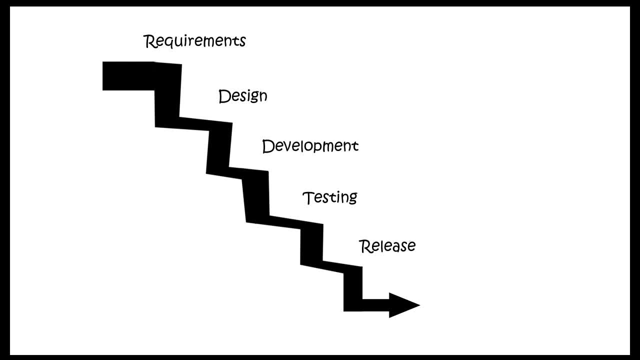 move forward, let's say, from requirements to design, certain things come into play. so, number one, as i mentioned, the team is going to change. the team dynamic needs to change. you need to make sure that you have the right players in place and the right roles filled. so it's no longer so. 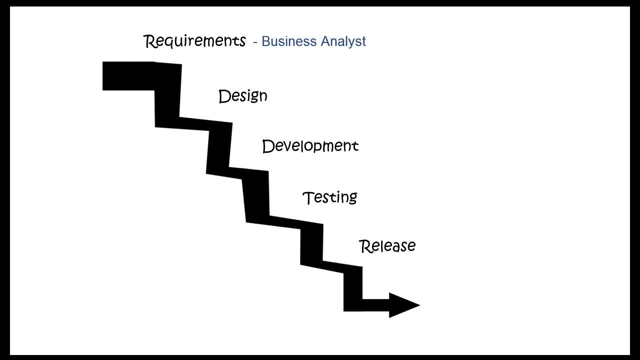 important to have a business analyst working with the business, determining the functionality and the business requirements, but now we need a system analyst who can actually help to do the right thing, and so that's where the analysis and design- and we have other videos out there on analysis and design- uml is a big part of the analysis and design process. for instance, uml. 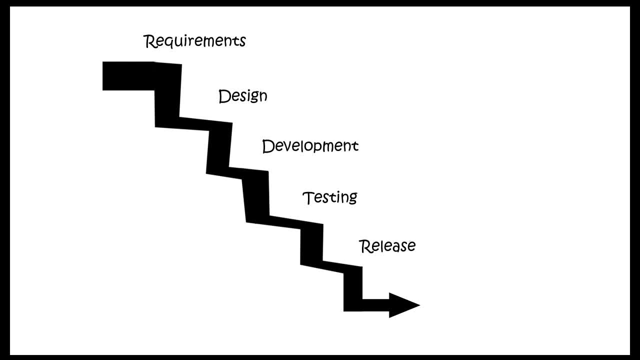 allows you to take your requirements and to elaborate them, using pictures and using notation, into a final physical design that you can hand over, that developers can use to have a when you move down from one level to the next, and this picture should hopefully allow you to see that and- and that is- it's easy to move from one level to the next. 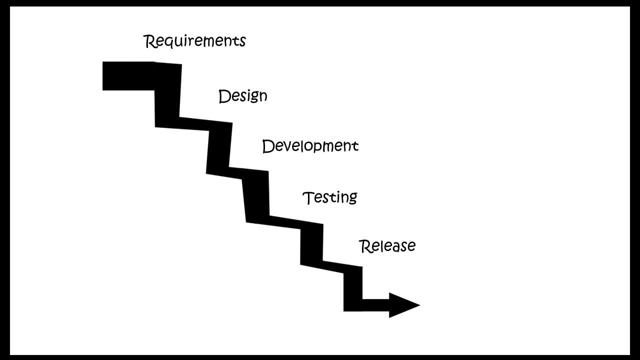 a lot of things have to happen when you move from one level to the next. each of these levels, each, each, each threshold between these levels, each step itself represents a milestone. so when you move down to the next level, you've passed that milestone. so in between each of these phases, in between requirements and design, there's the milestone of requirements being 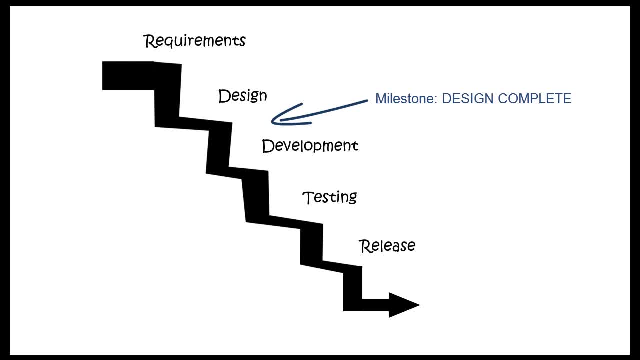 completed. in between design and development there's the milestone of design completed, and so on, so forth. so we assume that requirements are completed when we move from the top level to the second level. now we all know, anybody knows that requirements. they're never complete. you can't, you. 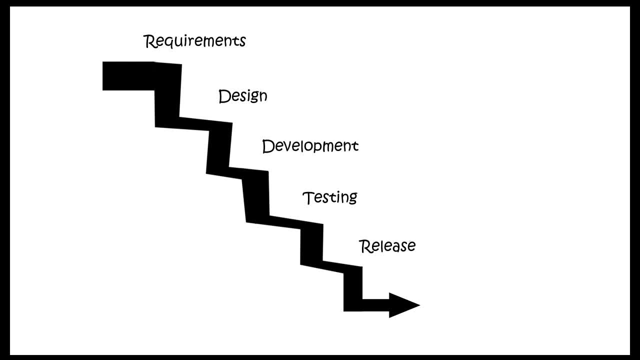 know. imagine you're saying again and again and again, you're saying: this is a интересно chapter. you need to know sovereignty and time and this is a round. this is the hiking, which is an own, I always emphasize. a negative goal Is to be a very expensive one. Those are all considerations to help you determine. 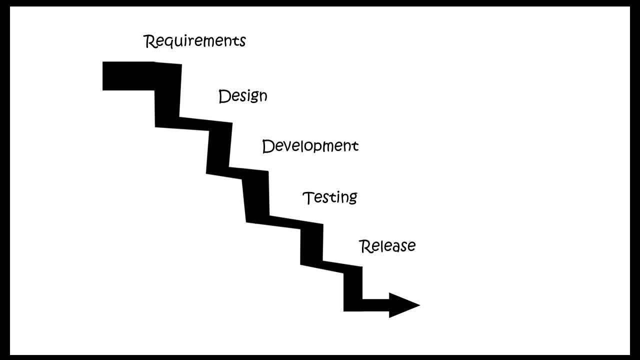 whether or not that the waterfall life cycle is appropriate for the project. So once I move from requirements to design, the requirements are complete. They've been signed off. We've passed this milestone, so we've gathered all these stakeholders together and we've reviewed the requirements. 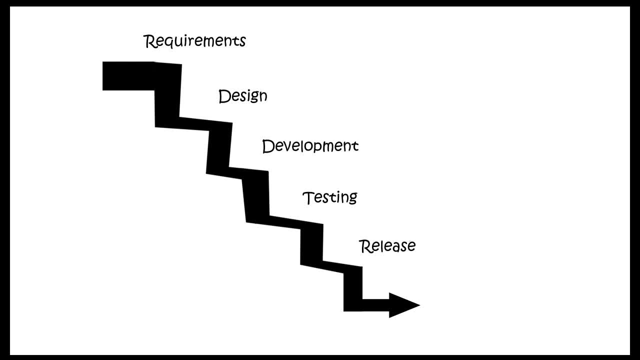 Everybody agrees the requirements are thorough and done, and at this point there is an agreement. We don't move forward thinking the requirements are not done. The waterfall is very prescriptive as far as that is concerned. Once requirements are done, then we can move to design. And then we encounter: 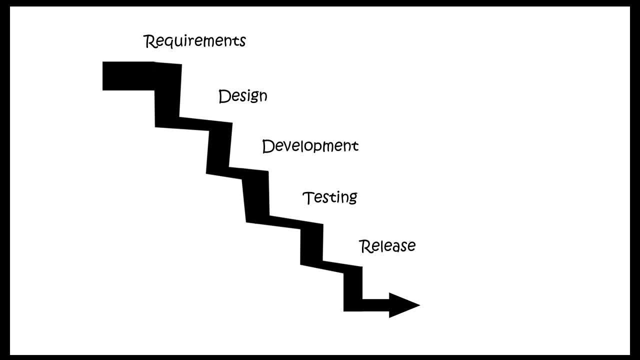 this strange aspect of the waterfall model that really makes it somewhat inflexible. So now we're down at design with the assumption that requirements are complete And we move forward. We change the team, We bring on new players. Some of the team members might move on a bit. The business analysts are no longer. 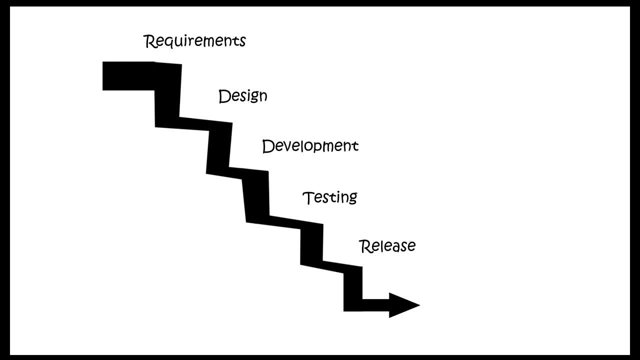 going to be so busy. They're not going to be building that business requirements package, The product people again might not be working so heavily and needing to provide so much information for the project to proceed. We've handed it over now to the system analysts in the development team, because the system 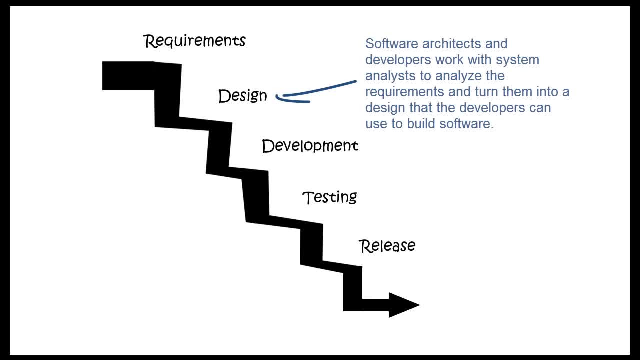 analysts and the developers are the ones who do the design, Which means again that the team dynamic is changing. The way that we're billing the team is different. We have we have a different set of players here That you know. we've made some.